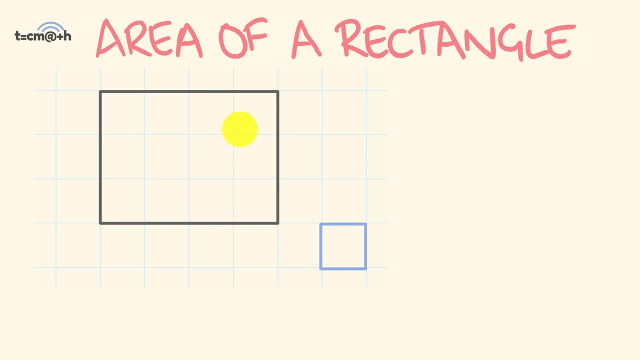 dealing with a two-dimensional shape. A two-dimensional shape is a flat shape that has two dimensions. A rectangle has the dimension of length and it has the dimension of width. So when we're looking at describing the area of this two-dimensional shape, we need to use 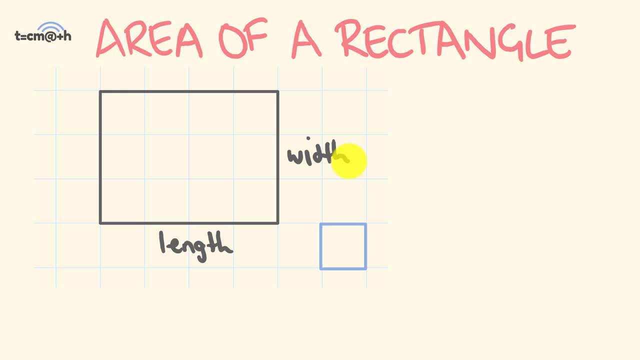 special two-dimensional units, Square units such as we have here, say in the forms of, say, meters squared, So this could be one meter squared, which is literally going to be one meter by one meter. It's a two-dimensional unit that we can use to describe the space taken up by a two-dimensional. 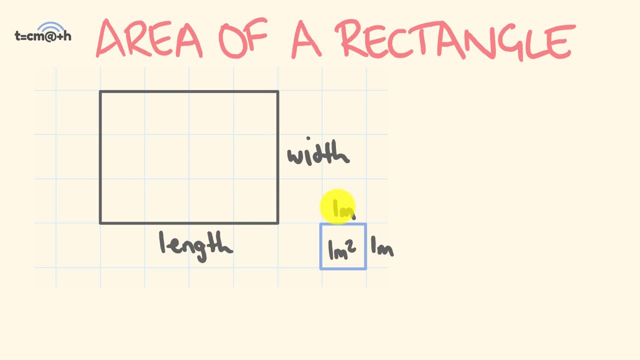 shape. We could also have centimeters squared, which would be one centimeter by one centimeter, or inches squared, which would be one centimeter by one centimeter. So this is a two-dimensional unit, one inch by one inch. I think you get the idea on that. So how do you go about working out the 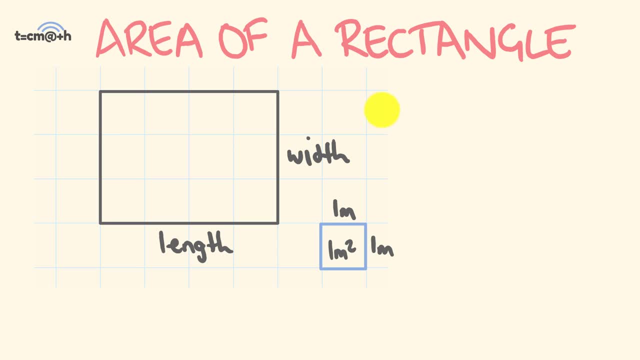 area of a rectangle. Well, the formula is pretty simple for this: The area of a rectangle is equal to the length multiplied by the width. The length times the width. Okay, so pretty simple. So, pretty simple. Let's put a couple of dimensions in here. So here we have three meters. Okay, one, two, three. 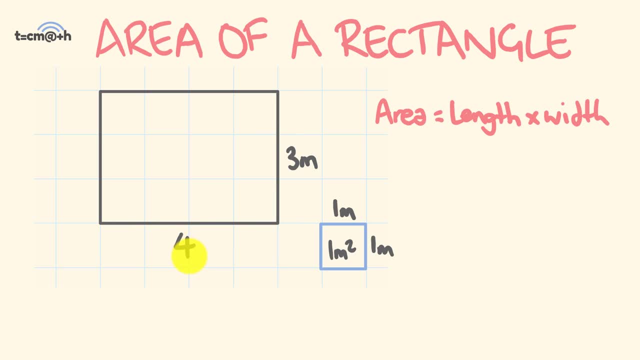 meters and along our length here We have four meters. So the area is equal to the length times the width. The area is equal to the length, which is four meters, multiplied by the width, which is three meters. Four meters times three meters is equal to 12 meters squared. Okay, meters times meters gives us meters squared. 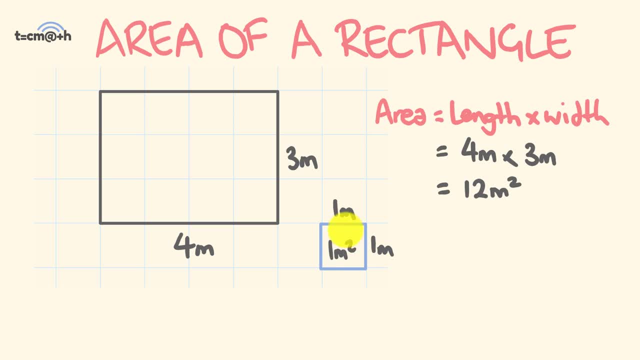 Same way here. Meters times meters gives us meters squared, And we can see that this is the case. You can see how many one meters squared occur in our rectangle. here We have one, two, three, four, five, six, seven, eight, nine, ten, eleven, twelve. So it's. 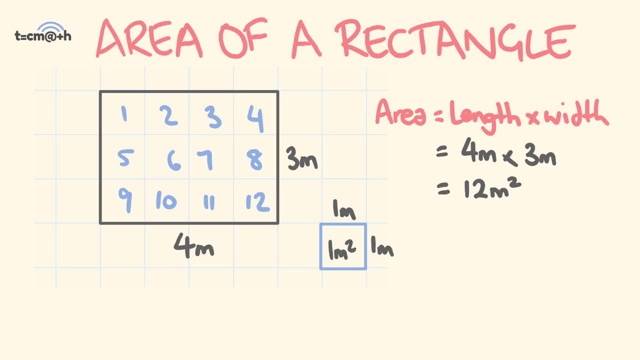 pretty simple, little thing to do, right? Just one thing to watch out for, and I'll show you in this example right now. Okay, in this example here, we are going to work out the area of a rectangle that has a length of three thousand millimeters and a width of 2.5 meters. But you might notice a 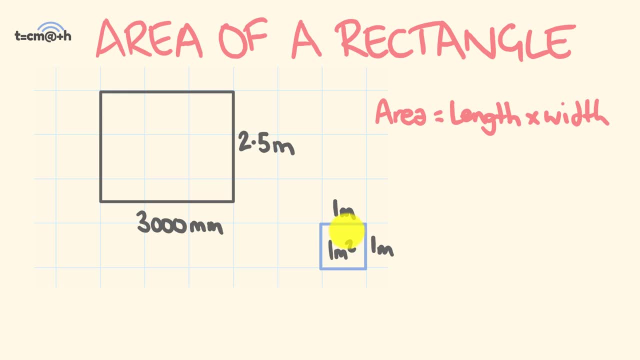 little bit of a difference here. We're going to be trying to work this out in meters squared, But we have this problem. We have a unit here that's in meters, but our unit here is in millimeters. So it's an important thing that when you're working out area, that you're dealing with the same units. 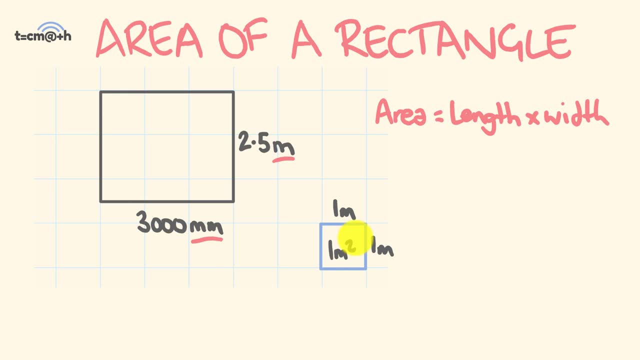 And in this case, because we want things in meters, we're going to start with our units both being in meters. So this one here is already in meters, but our three thousand millimeters needs to be changed across two meters. Now, you may or may not know this, but there is one thousand millimeters. 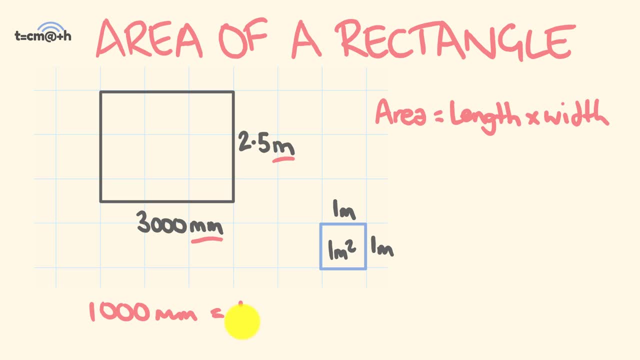 in weight. So that's a lot of weight. So we're going to work this out in meters squared And we're going to get one meter. So how many meters in three thousand millimeters? This is equal to three meters. We divide by a thousand and get three meters. So now we can work out this area, The area. 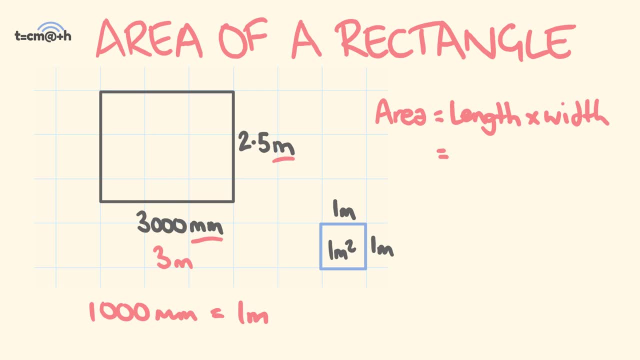 is equal to the length times the width. The length is three meters, The width is 2.5 meters. So three times 2.5, we have an area which is equal to 7.5 meters squared. Okay, here's the final example. 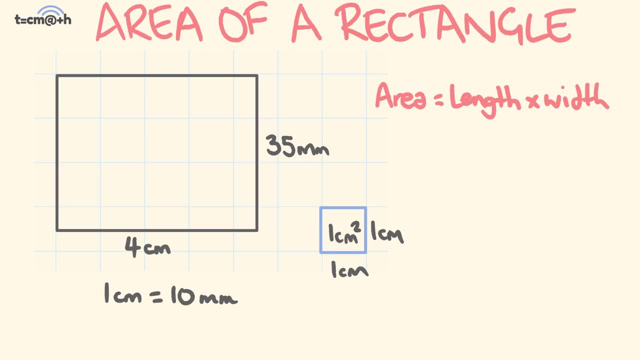 You give it a go. What you're going to see is we have a rectangle which has a length of four centimeters and a width of 35 millimeters, So we're going to work out the area. So, first off, what you're going to have to do is you. 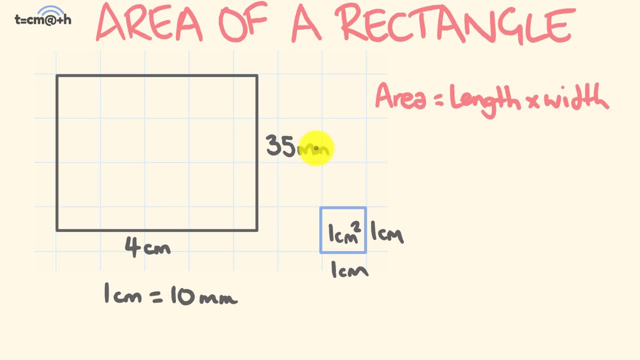 are going to have to change these millimeters here in two centimeters. There is 10 millimeters in a centimeter, So this is 3.5 centimeters. Now we can go through and work out the area. The area is equal. 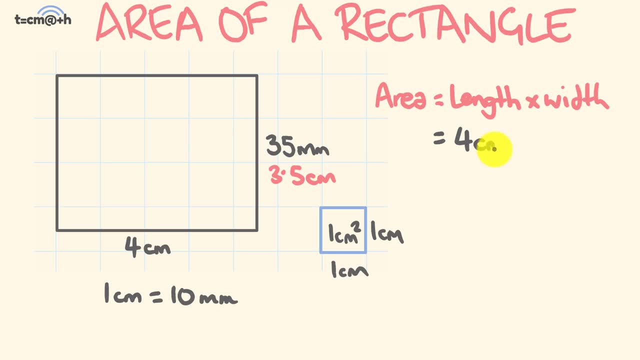 to the length, That is four centimeters, Multiplied by the width, That is 3.5 centimeters. Four centimeters times 3.5 centimeters is equal to 14 centimeters squared. Anyway, that's my quick video looking at how to work out the area of a. 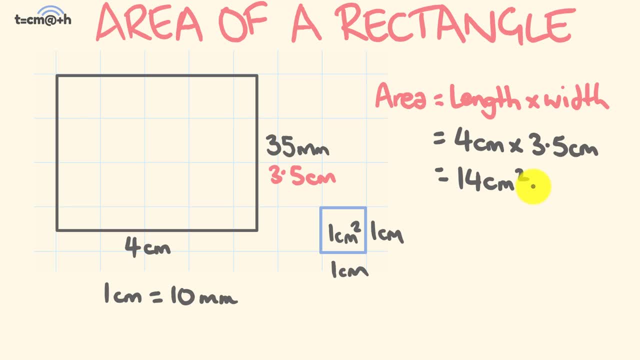 rectangle. It's pretty simple, but it's a pretty simple thing to do. Anyway, tell us what you thought of this video. Please like and subscribe. See you next time, Bye. Captions by GetTranscribedcom.